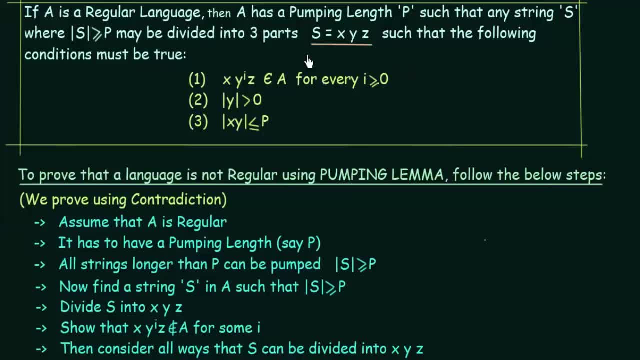 So here we have the rules of pumping lemma. So it says that if a language is regular, then it need to have a pumping length, let's say p, such that any string whose length is greater than or equal to p may be divided into three parts: x, y and z. 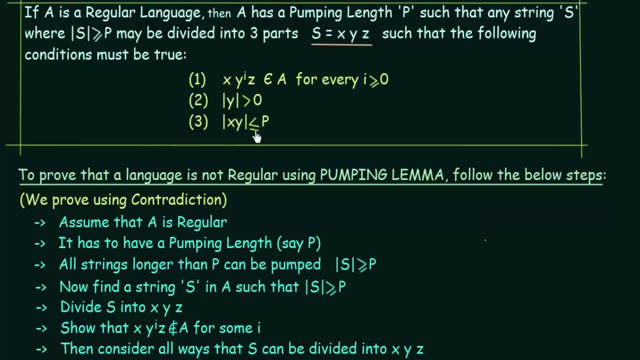 such that all these three conditions should be satisfied. So I have already discussed this in the last lecture, So I will not be discussing this again, So let us go straight to the steps that we need to follow in order to prove this. 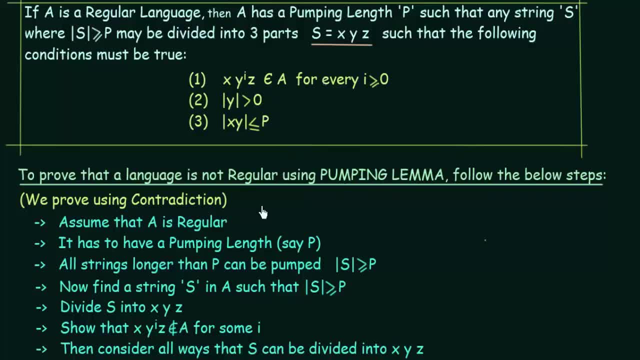 So, in order to prove a language is not regular using pumping lemma, the following steps are to be followed. First of all, we assume that a is regular, So we assume that the language which is given is regular. And if a is regular, then it has to have a pumping length which we will call p. 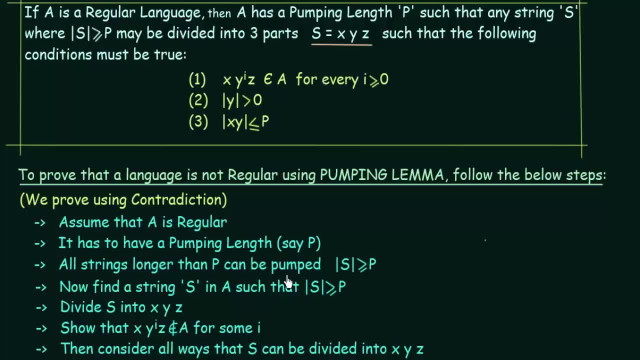 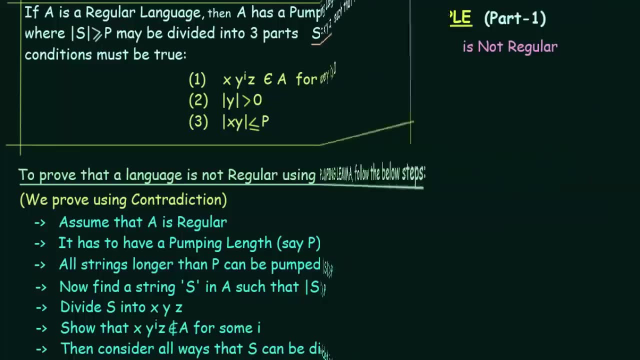 such that all strings longer than p can be pumped, And after that we will take a string s, such that its length is greater than or equal to p, and we will divide it into three parts: x, y and z. So let us do that. 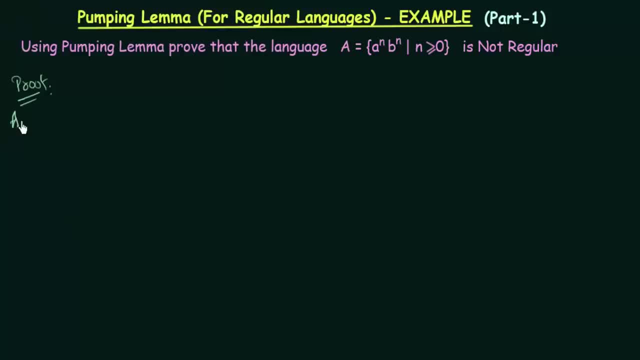 So the first step is to assume that a is regular. So we assume that a is regular. Now, if we assume that a is a regular language, then it needs to have a pumping length, And let me call the pumping length p. 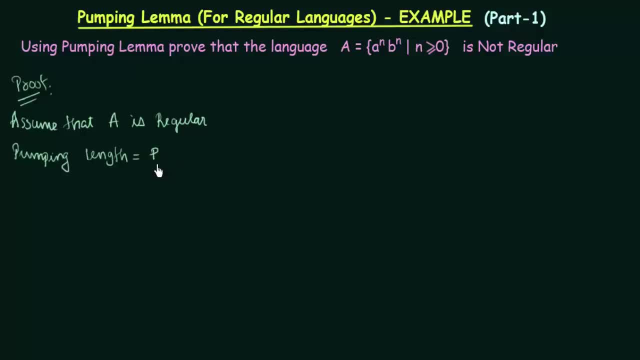 So we have a pumping length p, such that any string whose length is greater than or equal to p should be able to be pumped. Now let me choose a string which we will call s, And let us say that s is equal to a raised to p. 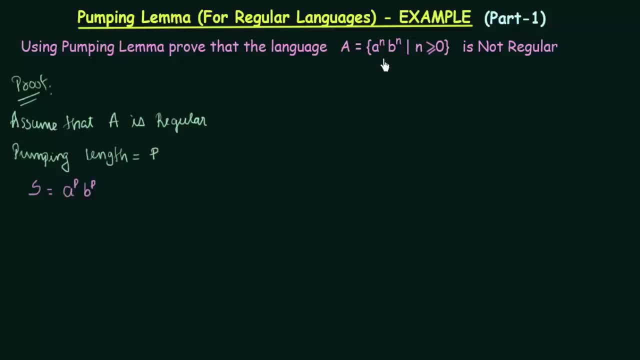 b raised to p, where p is the pumping length. A language is of this form, So instead of n, I am taking p, which is the pumping length. Now what was the next step? We need to divide this into three parts. 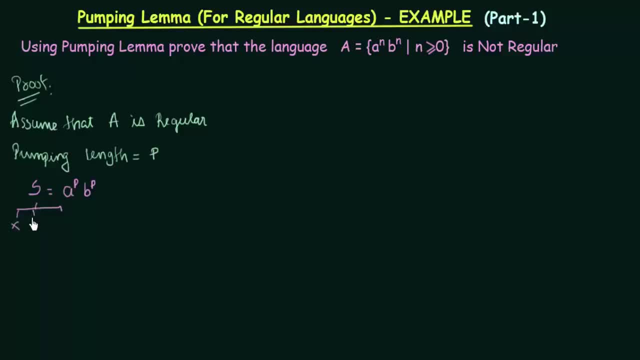 What are they? x, y and z. Alright, Now let us see how can we divide this into three parts: x, y and z. Now, let us see how can we divide this into three parts: x, y and z. Now, let us see how can we divide this into three parts: x, y and z. 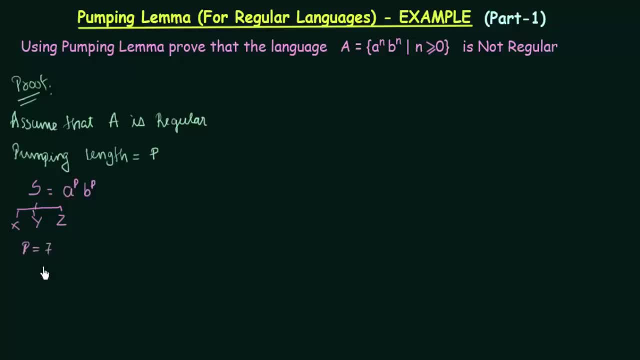 For now, let me assume that my pumping length is equal to 7.. Now, let me assume that my pumping length is equal to 7.. Now, let me assume that my pumping length is equal to 7.. Now I can write this string as: 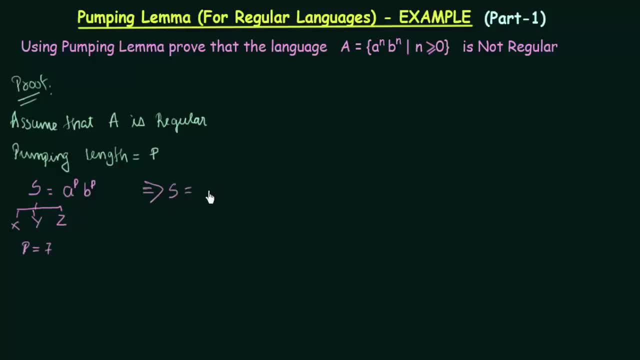 how can I write it? I can write: s is equal to 1,, 2,, 3,, 4,, 5,, 6,, 7, a 7 times, followed by 1,, 2,, 3,, 4,. 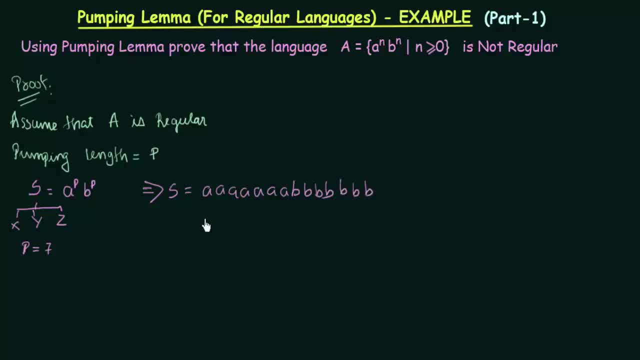 5,, 6,, 7, b, also 7 times. Okay, Assume that this is our string, which has pumping length of 7.. Now let us see all the possible ways in which we can divide this S into three parts: x, y. 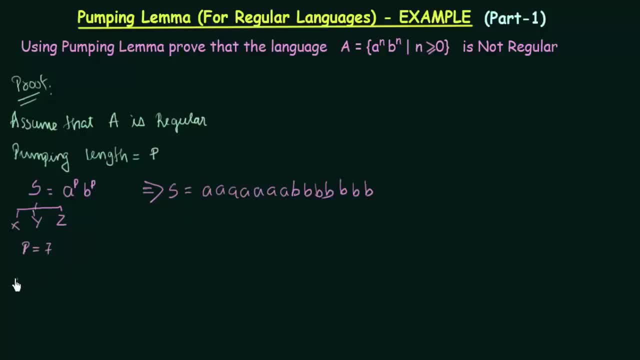 and z. So for that, let me take first case, Case number one. So the case number one is that the y part, that is, this y, is in the a part. What do I mean by this? You will be clear when I do this. 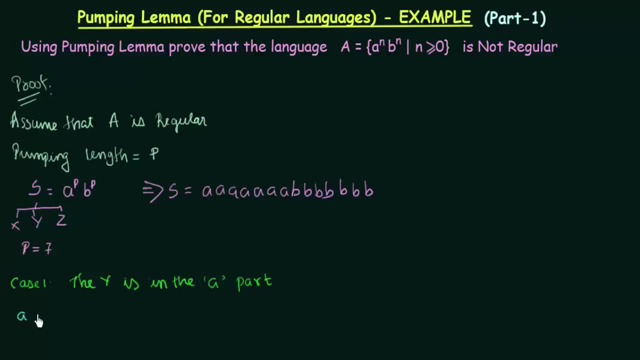 So what I mean by this is, let us say, we have like this: 1, 2,, 3,, 4,, 5,, 6, 7 and 1, 2,, 3,, 4,, 5,, 6, 7.. 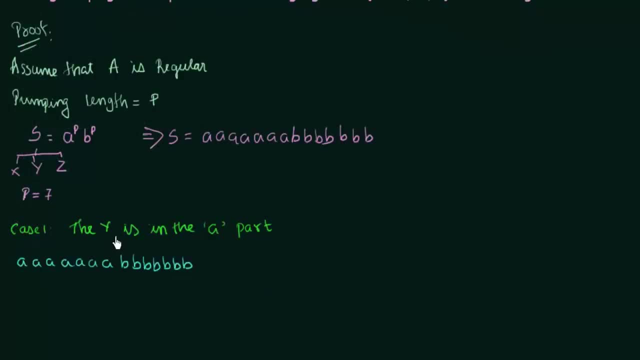 Okay, so this is my string and the y is in the a part. So what I mean by this is: let us assume that y is this one, This part. Okay, So if this is y, this will be x and the remaining from here to the end, this will be z. 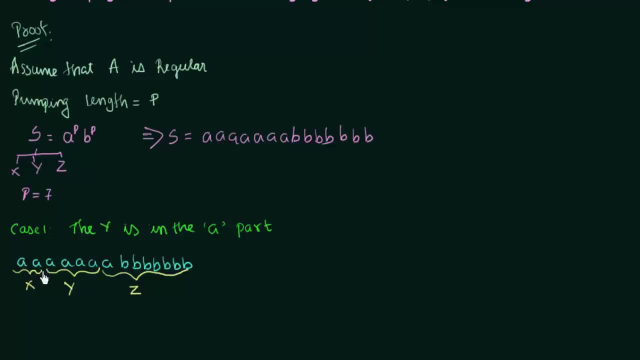 Okay, So this is the first case. So we have divided it into three parts: x, y and z, and then the y part, the middle part it is in the a part Means it contains all a's, a, a, a, a. these four a's. 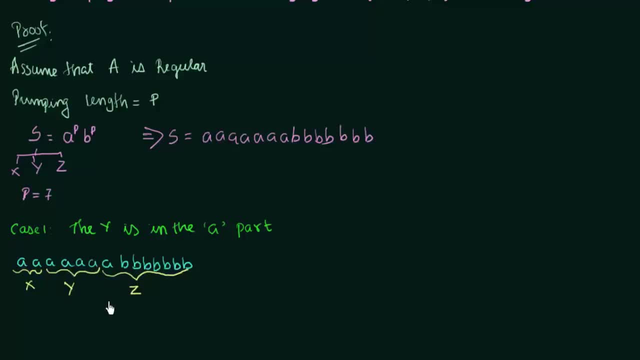 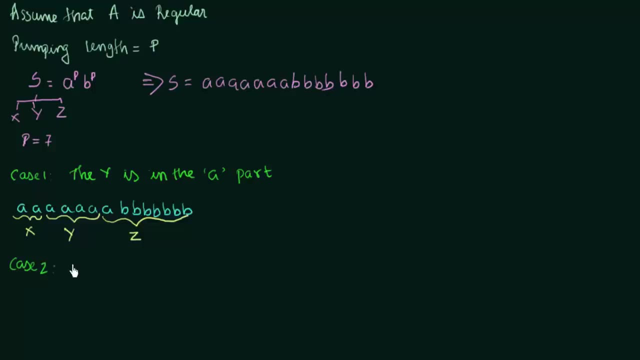 So this is how I can divide it in one way, And there is another way we can divide. How is that? Let us see Case number two. Case number two says that the y is in the b part. The y is in the b part. 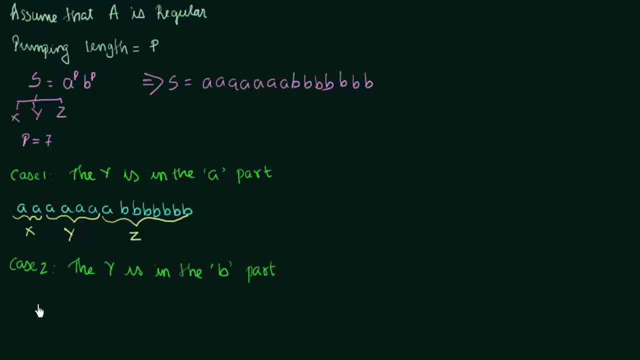 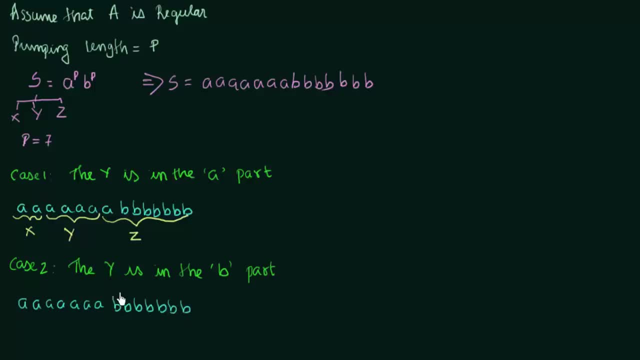 1, 2,, 3, 4, 5, 6, 7.. So now I will divide it in such a way that the y is in the b part. For that let me take these four b's from here. 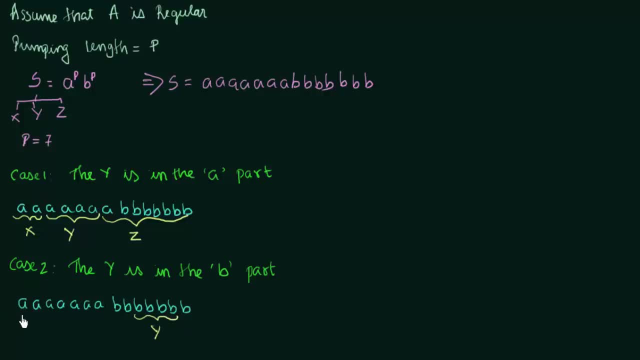 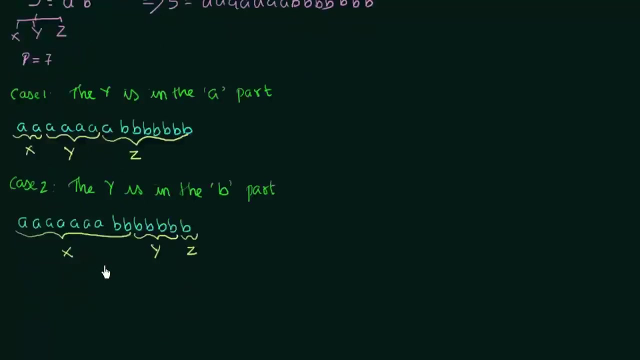 Okay, This is my y, And then this whole part. this is x and this one will be z, So y contains only b. That is the case number two. Now case number three. There is one more case that we can have. 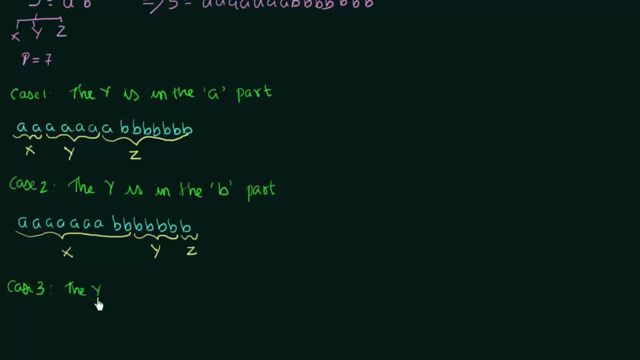 Case three. It says that the y is in the a as well as b part. Now, how is this? I hope you already guessed it. It is like this: 1, 2,, 3,, 4,, 5,, 6, 7.. 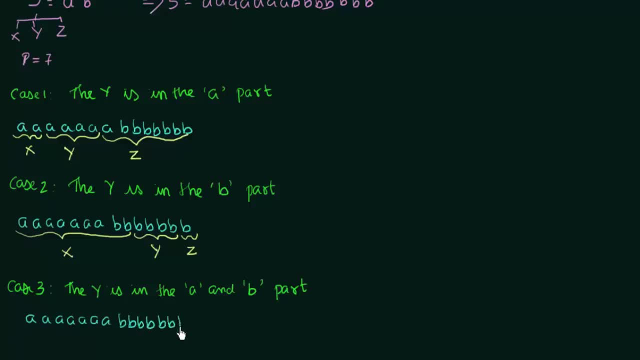 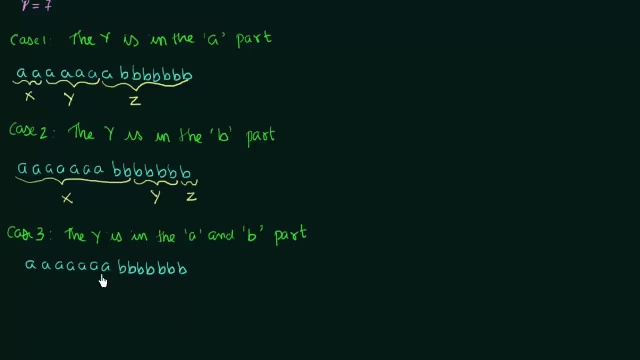 1,, 2,, 3,, 4,, 5,, 6, 7.. Now for the y to be in the both a and b part. I will choose this to be my y: 2 a's from here, 2 b's from here. 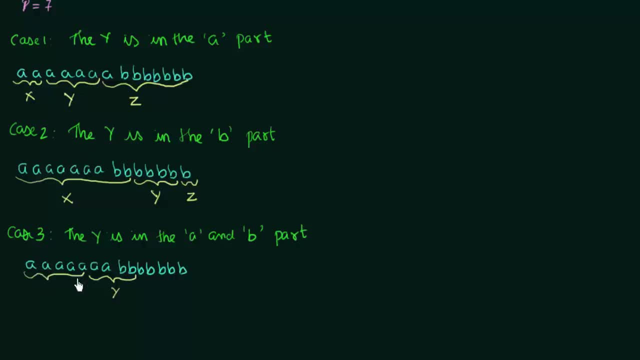 This is y And this is x and this is z, So y has both a and b. So that is case number three. So these are the three possible ways in which the y is in the a and b part. Okay, So these are the three possible ways in which we can divide our string into three. 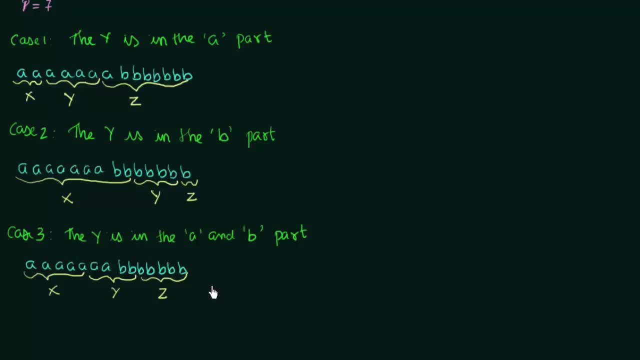 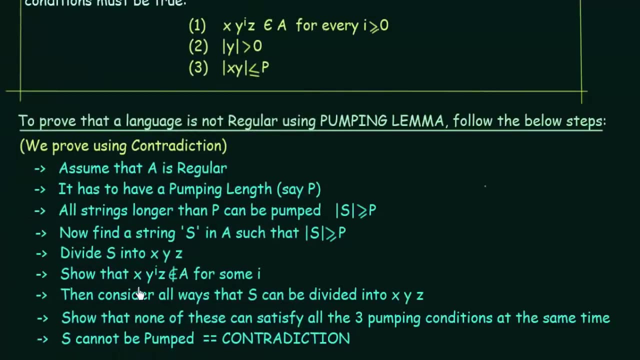 parts x, y and z. Okay, Now what do we have to do? Let us just go back and look again. So we have divided s into x, y and z. Now we have to show that xy raise to i. z does not belong to a for some i. 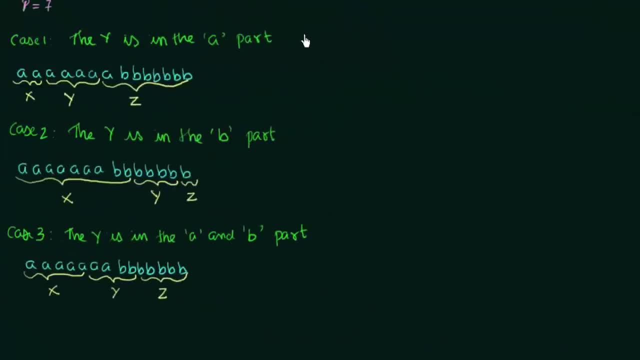 So let us do this Okay. So, coming to the first case, let me draw a line here and let us do this Okay. case number one: so the for the first case, let's take any X, Y, I, Z. so here, let 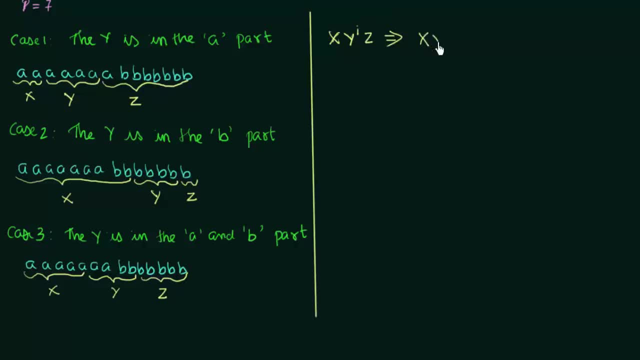 me. take my I to be 2. that means X, Y square Z. that means I have to repeat my Y part twice. so this is the first case I am looking at. so what is my X? X is a, a and what is my Y? Y contains 4 is 1, 2, 3, 4, and I have to do it twice. that means 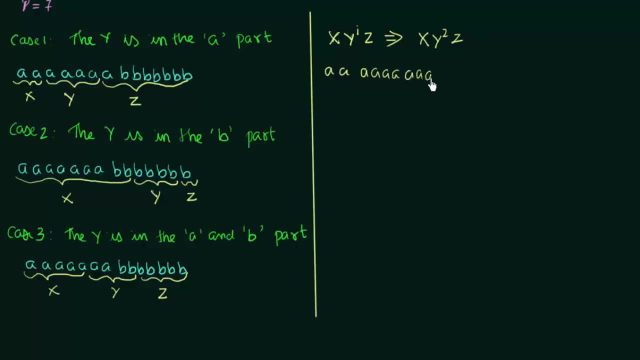 again I have to repeat Y: 1, 2, 3, 4. all right then Z. Z contains 1 a and 7 B's: 1 a and 1, 2, 3, 4, 5, 6, 7. okay, so we get this string. now we have to. 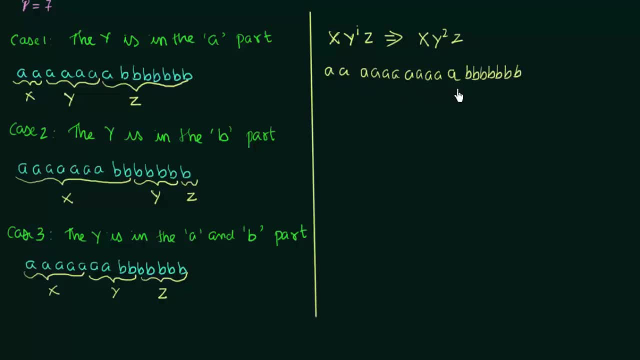 see the first case number one. so this is the first case number one. so we have to see the first case number one. so this is the first case number one. so we have to see if. does this string lie in our language, a or not. so let us count how. 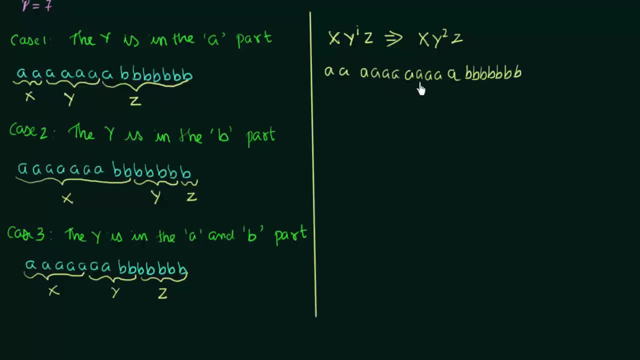 many is. we have your: 1, 2, 3, 4, 5, 6, 7, 8, 9, 10, 11. we have 11. is in how many B's? 7 B's, so 11 and 7. so the number of A's and the number of B's are not equal. so in our 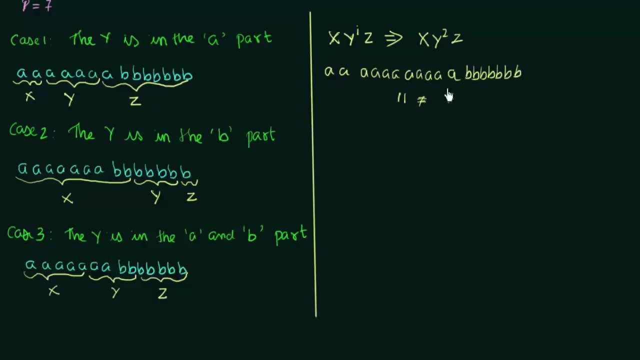 language, number of A should be equal to number of B's. so this string does not lie in our language. all right, this string does not lie in our language for case number one. now let's try the same thing for case number two. let me take X, Y raised to I. 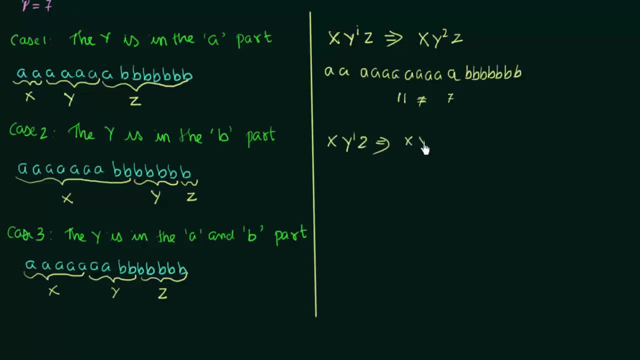 Z, and let me choose my I to be 2, so I have X, Y square Z. and what is X? X contains 7 A's and 2 B's, 1, 2, 3, 4, 5, 6, 7 and 2 B's and Y. Y contains 4 B's: 1, 2, 3. 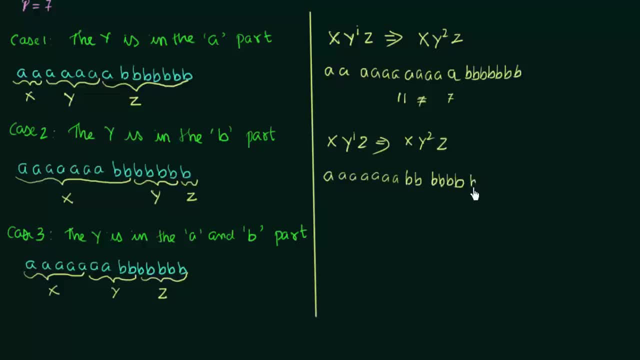 4 and I have Y square. that means I have to repeat Y once more: 1, 2, 3, 4 and then Z. Z is only 1 B. now let's count again how many S and B's we have. we have 1, 2, 3, 4, 5. 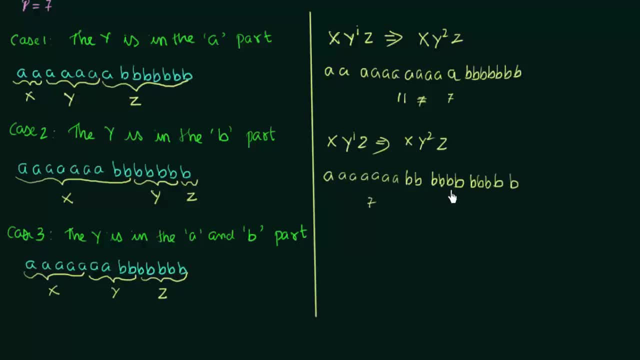 6, 7 A's. and how many B's? 1, 2, 3, 4, 5, 6, 7, 8, 9, 10, 11. we have 11 number of B's. again, the number of A's and B's are not equal, so even this does not lie in our language. 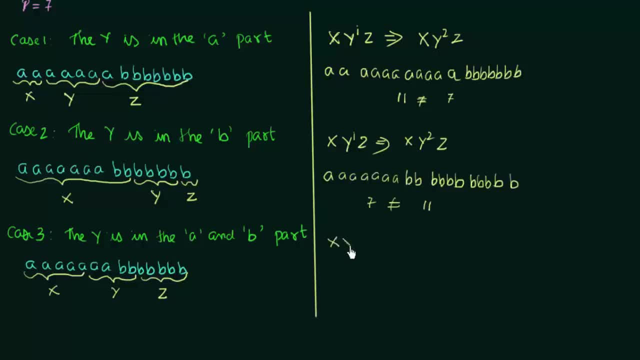 all right, so let's count again. do the same thing for case number three. I take S Y I Z and I choose my I to be 2. now let's see here: X is 1, 2, 3, 4, 5 A's, 1, 2, 3, 4, 5, and Y contains 2 A's and 2 B's. 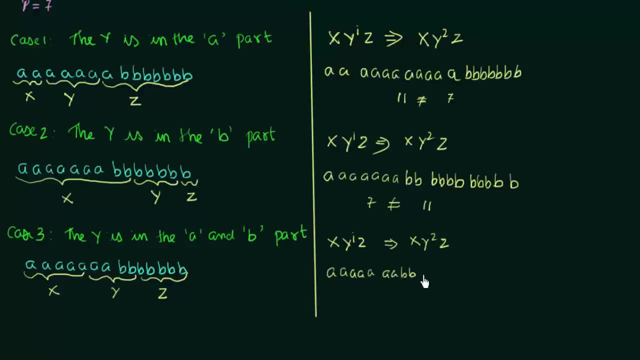 2 A's, 2 B's, and if you repeat Y once more, 2 A, 2 B and then Z, Z contains 1, 2, 3, 4, 5 B's. 1, 2, 3, 4, 5, 16, 7 A minus Z plus 2 A minus 2 H times a times 3 X square. 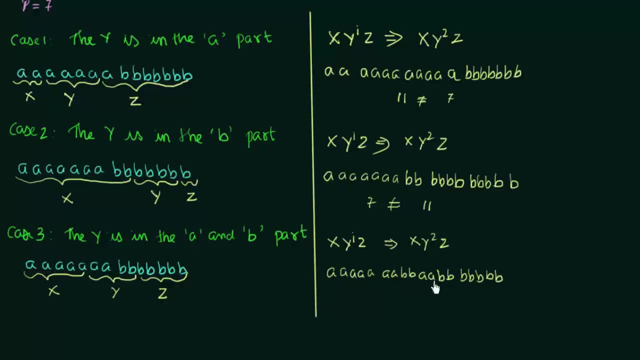 and add 4 to this. next: 1, 2, 3, 4, 5 B's: 1, 2, 3, 4, 5. so here, if you before we count, you can see that this does not follow the pattern. a raised to n, B raise to n. see here we have S and followed by two B'S and again. 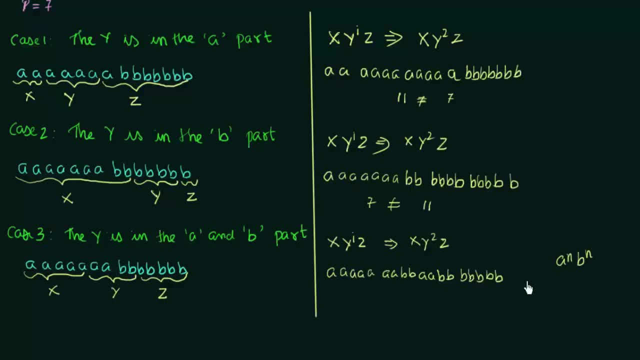 there are s NB, so it is not following this pattern. so this also does not like in our language. so we proved that when we take X, Y, I, Z and take another award like that power, before we enter into another, coordinate on the chilled C line left and right and right in. remember, remember, remember, right now, this is incorrect. it should be e divr into a squared. 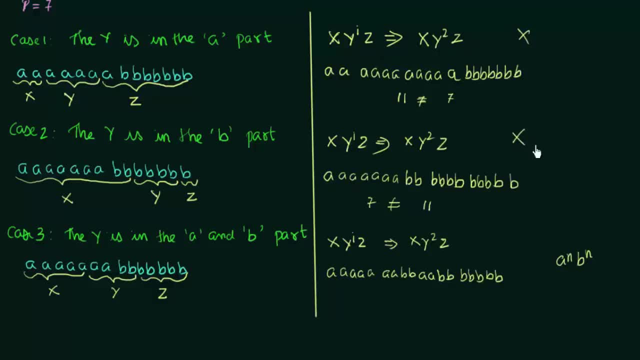 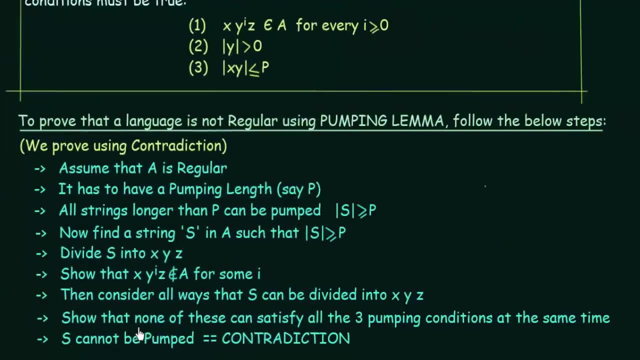 i to be 2. all this does not lie in our language, so let us turn back to our rules once more. show that none of this can satisfy all the three pumping conditions at the same time. so we saw that this condition cannot be satisfied, so we have taken X, Y, raised to. I said and we showed. 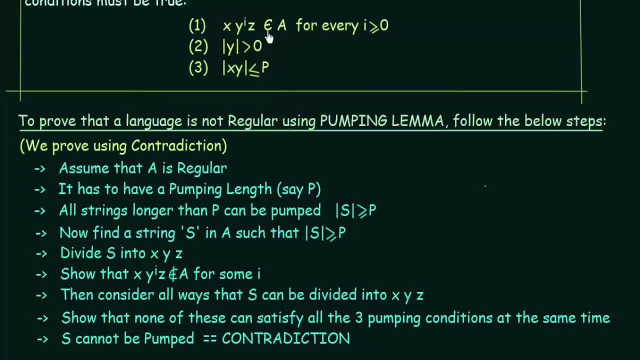 that it does not belong to a. so it will be regular only when it belongs to a. so we have shown that it does not belongs to a, hence it is not regular. so we can also show that these conditions are also not satisfied. let us see condition number three. condition number three says that length of X, Y 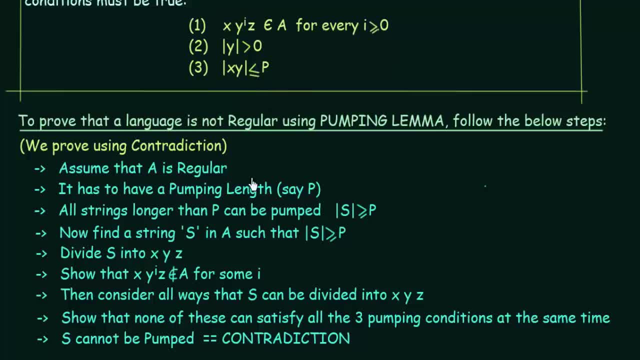 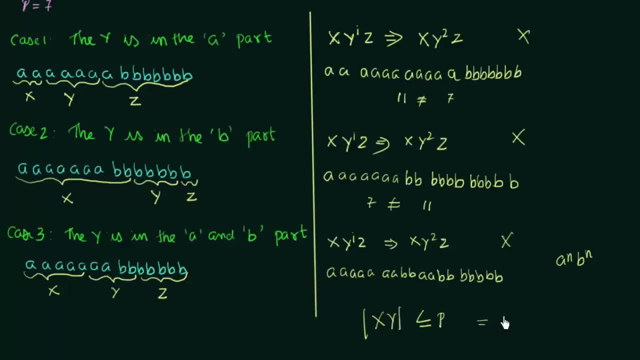 should be less than or equal to P. let us see if that was satisfying. or length of X, Y should be less than or equal to P, and in our case P was, P was seven. so let us see, in case number one, what is the length of X and Y together? one, two, three, four, five.